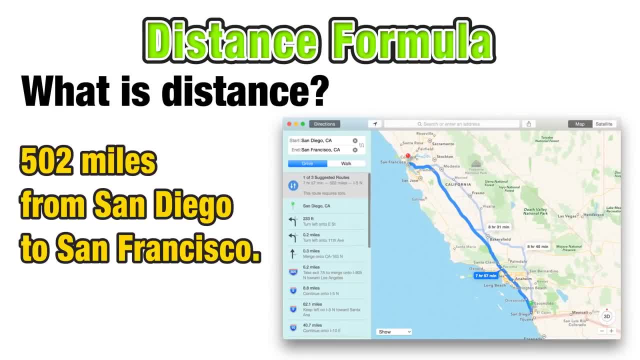 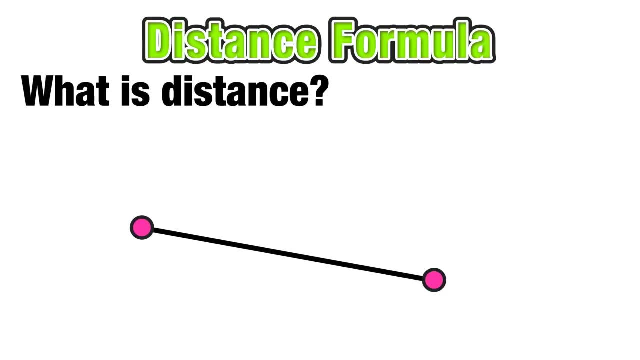 looking at distances between a starting point and an ending point. just like the drive from San Diego to San Francisco would be a distance of 502 miles, So for this lesson we're concerned with finding the distance between two endpoints connected by a line segment, in this case line segment CK. If we measured this line, 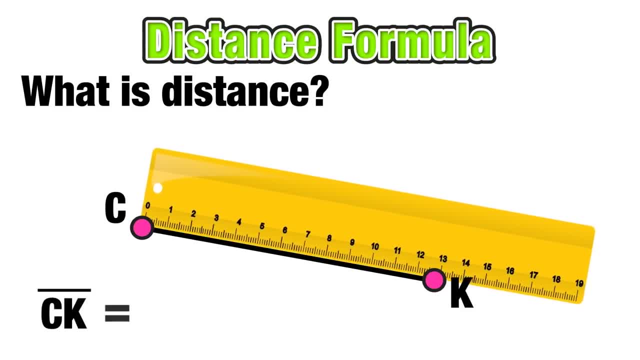 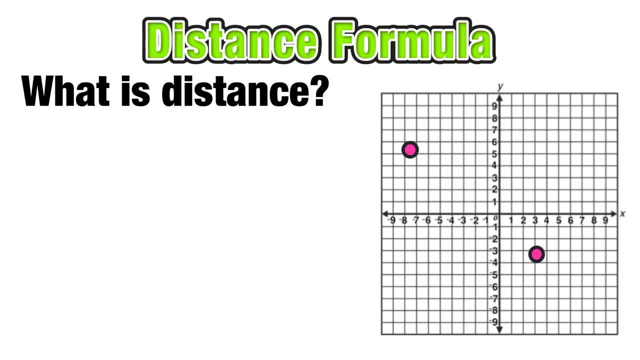 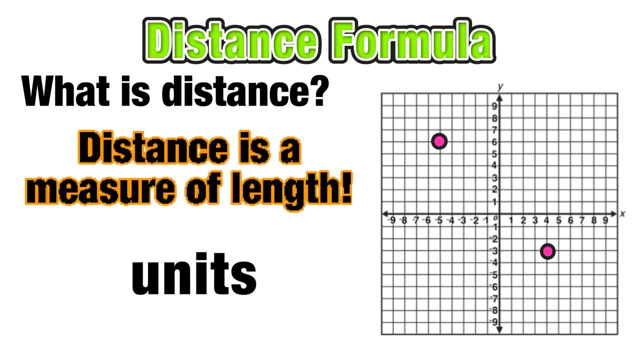 with a ruler, we could say that CK has a length of 13 centimeters, And we are going to extend this idea of finding distance between points on the coordinate plane. Please note that distance is a measure of length. the words are interchangeable. 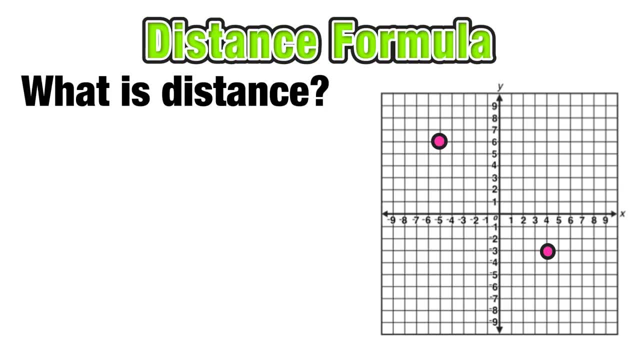 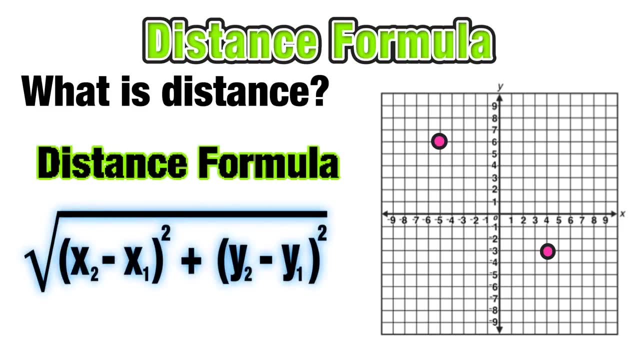 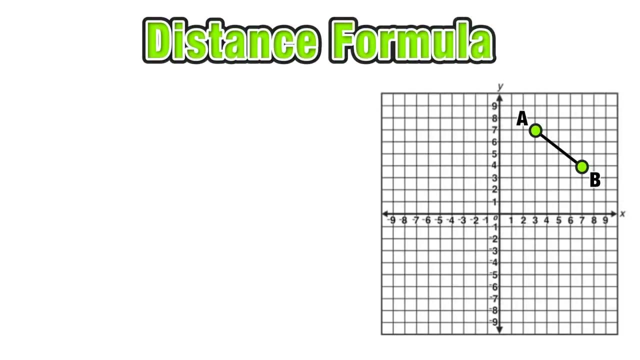 and distance is measured in units. Finally, when finding distances on the coordinate plane, our tool is not going to be a ruler, but the distance formula. So let's go ahead and learn how to use the distance formula. Our first example calls for finding the length of line segment AB. Now, when we see the word 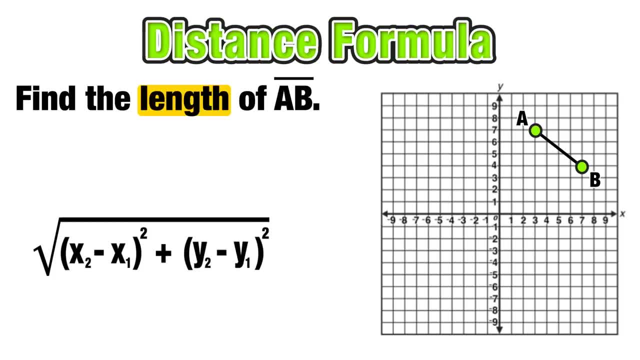 length. we should be tipped off to use the distance formula. First we are going to need the coordinates of the endpoints a and b, with a at 3,7 and b at 7,4.. Now again, a and b are both points with x and y coordinates, Since a is the first. 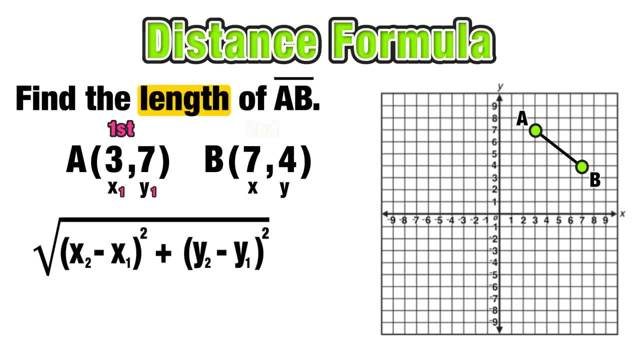 point, we will give it the ones, And since b is our second point, we should recognize these coordinates and use the distance point. we'll give it the twos: x2, y2. and now we're ready to use our formula. let's start off by looking at x1 and x2. x2 is 7, x1 is 3, so we have 7 minus 3 in. 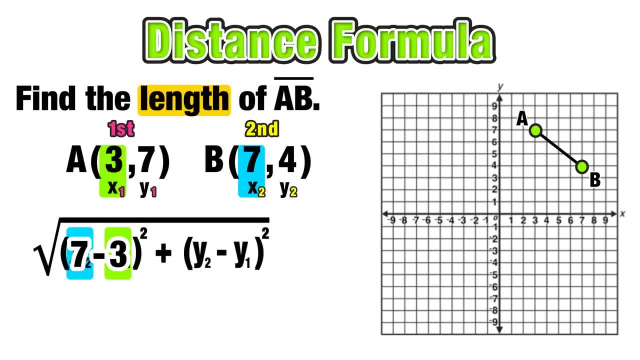 parentheses on the left side of the equation. now we can slide that over and look at y2 and y1. y2 is 4, y1 is 7, so we have 4 minus 7 in the parentheses on the right side of the distance formula equation. and now that we're done, 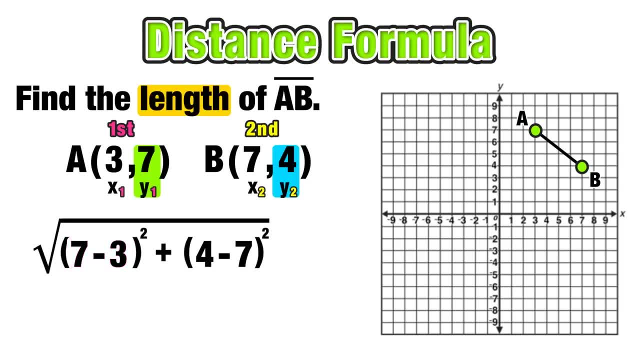 substituting, we can begin to evaluate. 7 minus 3, we know, is equal to 4. on the right side, 4 minus 7 is equal to negative 3. now we can evaluate the exponents: 4 squared is equal to positive 16 and we're adding that to negative 3. 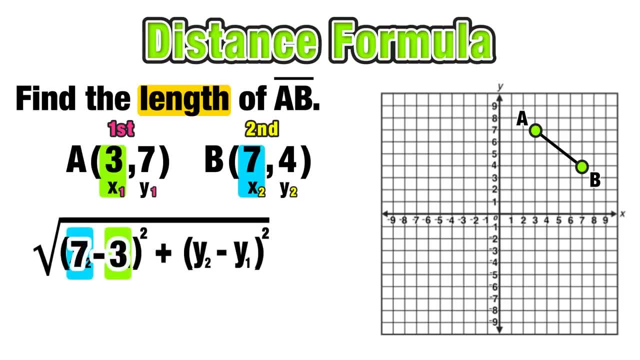 start off by looking at x1 and x2. x2 is 7, x1 is 3, so we have 7 minus 3 in parentheses on the left side of the equation. now we can slide that over and look at y2 and y1. y2 is 4, y1 is 7, so we have 4 minus 7 in the parentheses on the 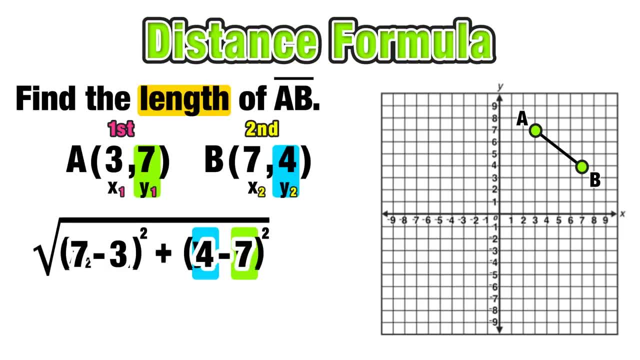 right side of the distance formula equation. and now that we're done substituting, we can begin to evaluate. 7 minus 3, we know, is equal to 4. on the right side, 4 minus 7 is equal to negative 3. now we can evaluate the. 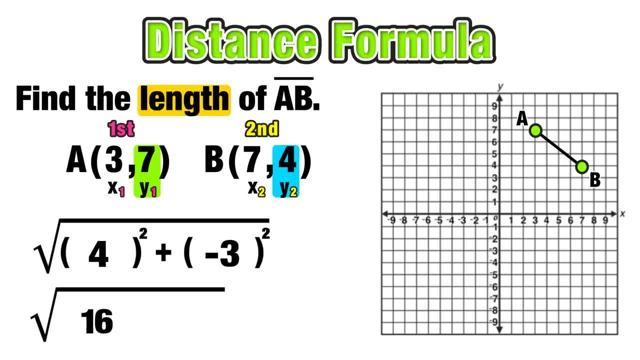 exponents: 4 squared is equal to positive 16, and we're adding that to negative 3 squared, which is equal to positive 9. remember a negative number squared is a positive value and we know that 16 plus 9 is equal to 25. 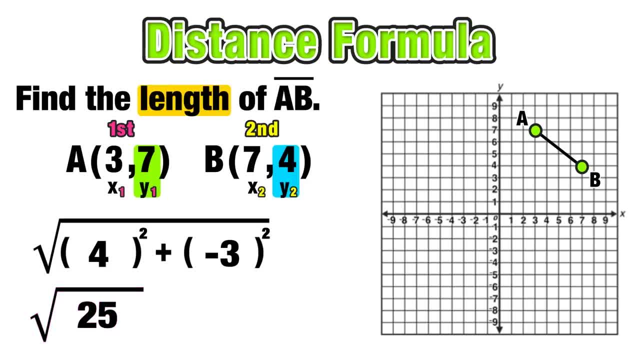 and finally, we can evaluate the square root. the square root of 25 is equal to 5. so what we just found is that line segment AB is 5 units long. now, real quick. if we look at AB as the hypotenuse of a right triangle, we notice: 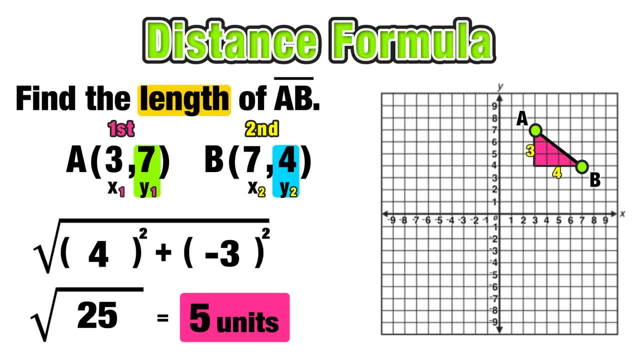 that the legs of the right triangle are 3 and 4. this is your classic 3, 4, 5 right triangle, and this value of 5 can also be found using the Pythagorean theorem. so we should see that the distance formula actually comes from the Pythagorean. 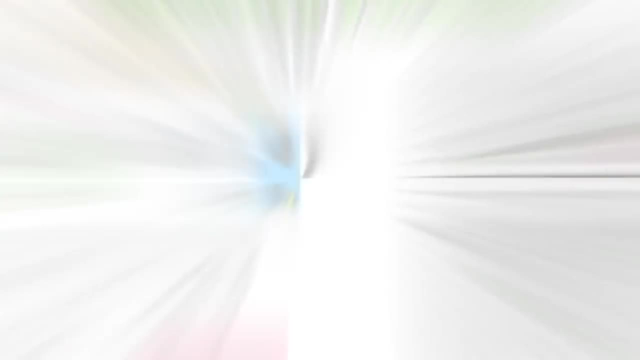 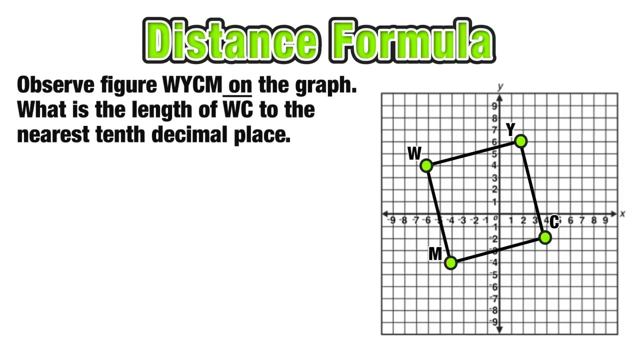 theorem: a squared plus b squared equals c squared. for our next example, we're going to be observing a quadrilateral on the coordinate plane with endpoints w, y, c and m. we want to find the length of line segment WC. so we know we're going to have to use the distance formula. again, notice that W and C are diagonal. 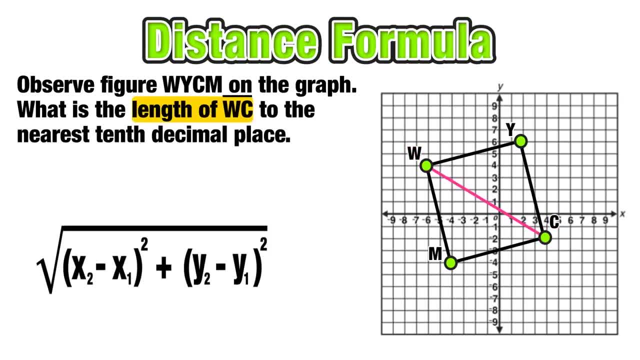 from each other. so this is a diagonal of this four-sided figure. so we have to construct that line to help us visualize what line segment WC looks like on the coordinate plane. now we can write down the coordinates of W at negative 6, 4, that's your x1, y1, and C at 4 negative 2, that's your x2, y2. in the distance, 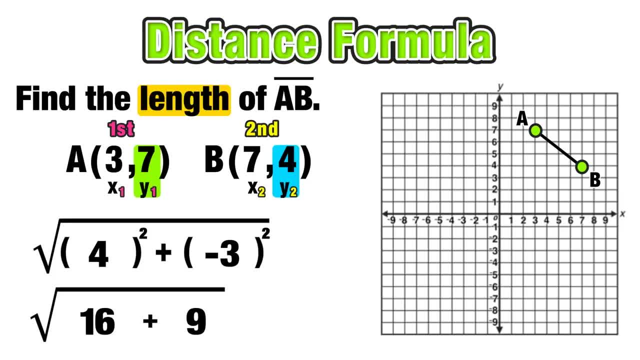 squared, which is equal to positive 9- remember a negative number- squared is a positive value and we know that 16 plus 9 is equal to 25. and finally, we can evaluate the square root. the square root of 25 is equal to 5. so what we just found is that line segment AB is 5 units long. 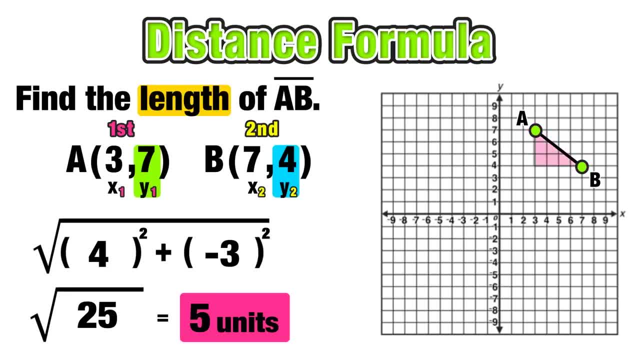 now real quick. if we look at AB as the hypotenuse of a right triangle, we notice that the legs of the right triangle are 3 and 4. this is your classic 3, 4, 5 right triangle, and this value of 5 can also be found using the Pythagorean theorem. so 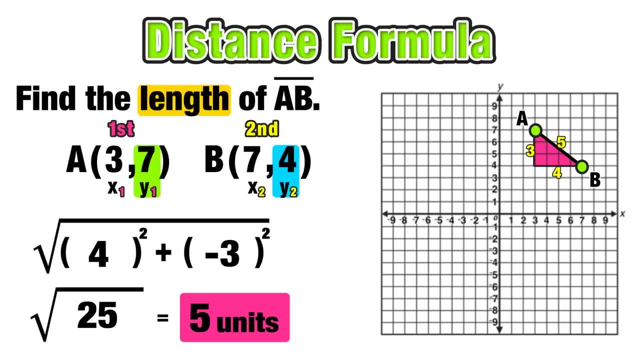 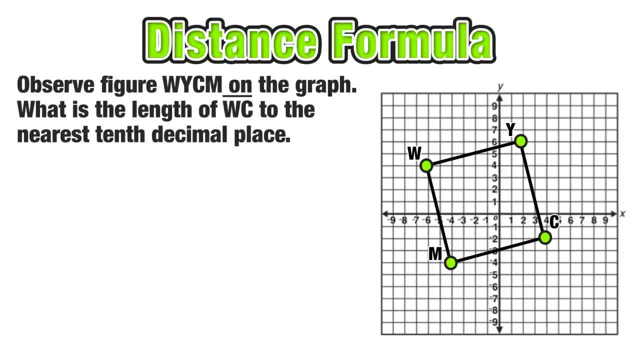 we should see that the distance formula actually comes from the Pythagorean theorem: a squared plus b squared equals c squared. for our next example, we're going to be observing a quadrilateral on the coordinate plane with endpoints w, y, c and m. we want to find the length of line segment WC. so we know we're going. 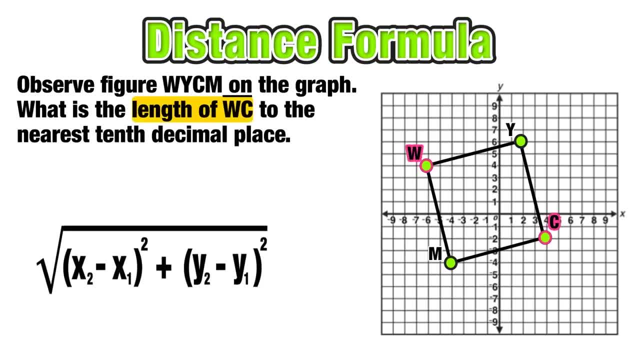 to have to use the distance formula again. notice that W and C are diagonal from each other. so this is a diagonal of this four-sided figure. so we have to construct that line to help us visualize what line segment WC looks like on the coordinate plane. now we can write down the coordinates of W at: 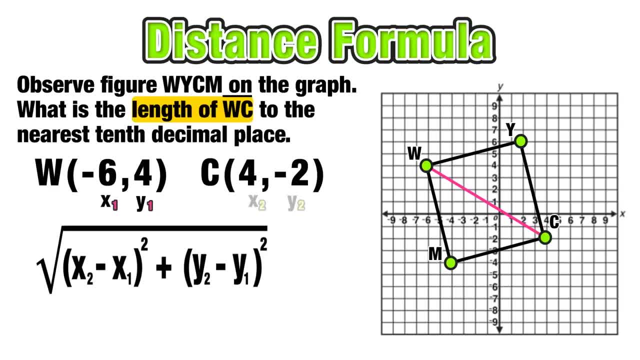 negative 6, 4, that's your x1- y1, and C at 4 negative 2, that's your x2- y2. in the distance formula we can now substitute: x2 minus x1 is going to be 4 minus negative 6. then on the right side of the distance formula, y2 minus y1 will be. 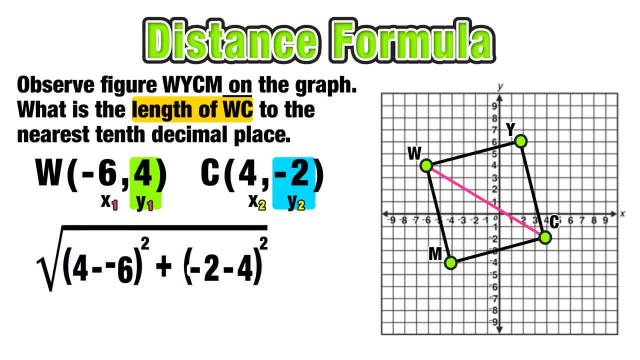 negative 2 minus 4. so now we can continue to evaluate 4 minus negative 6. the double negative becomes a positive. so 4 plus 6 equals 10 and on the right side of parentheses, negative 2 minus 4 is equal to negative 6. now the exponents 10 squared is equal. 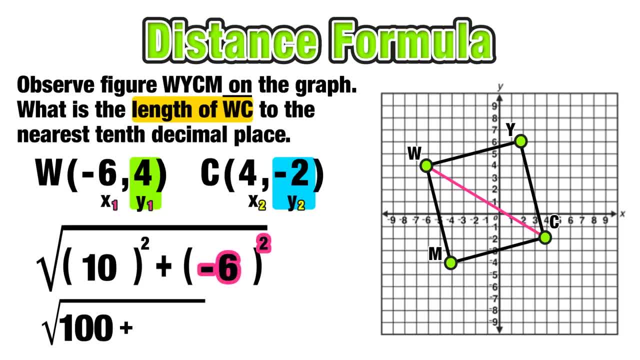 to 100 plus negative 6 squared is equal to positive 36, and 100 plus 36 is equal to 136. and now we just need the square root of 136, which is going to equal an irrational number. and since the question asks us to round to the nearest tenth decimal place,